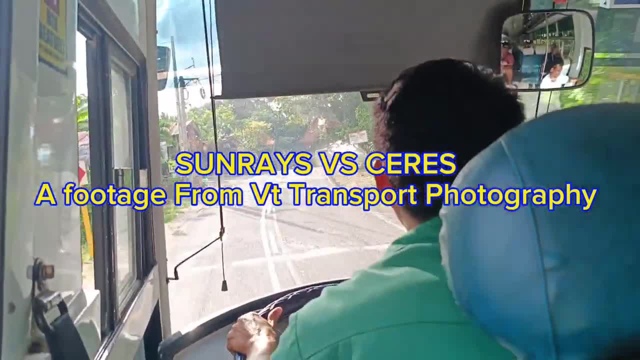 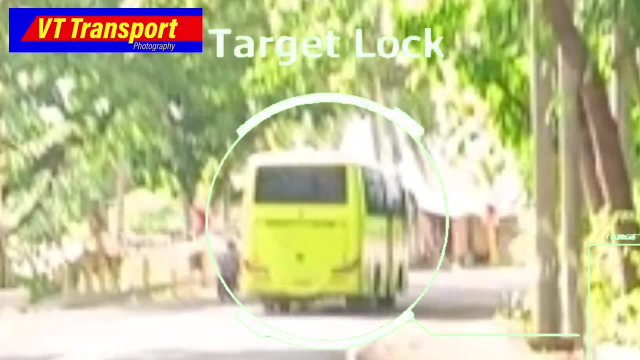 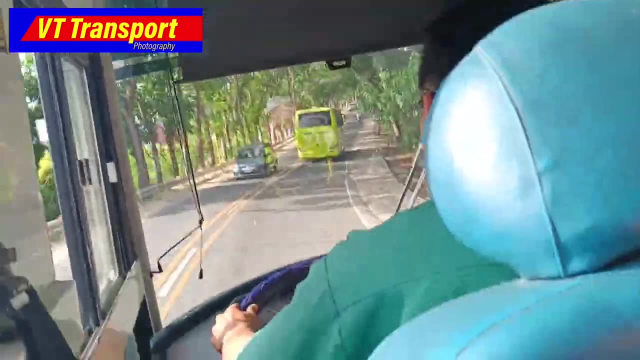 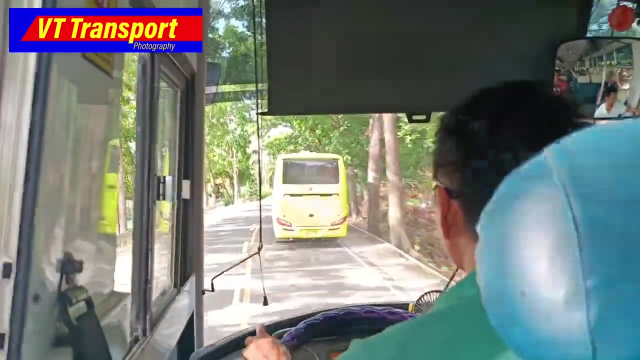 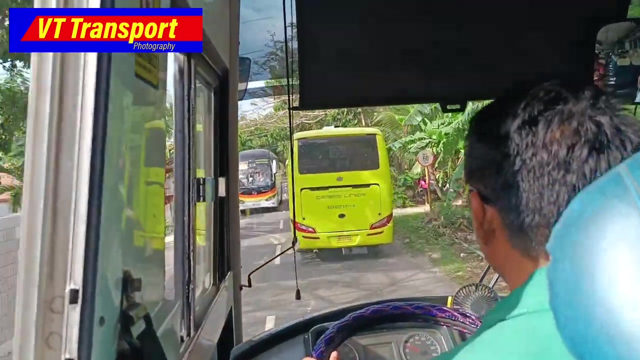 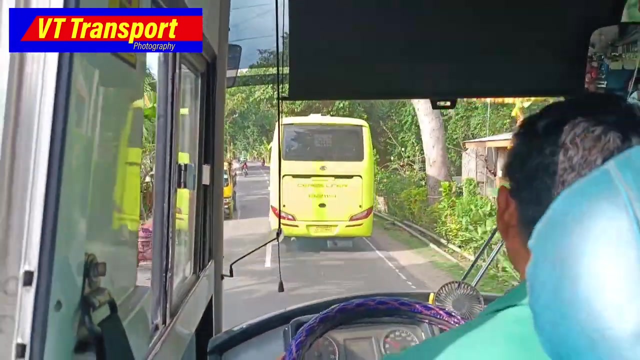 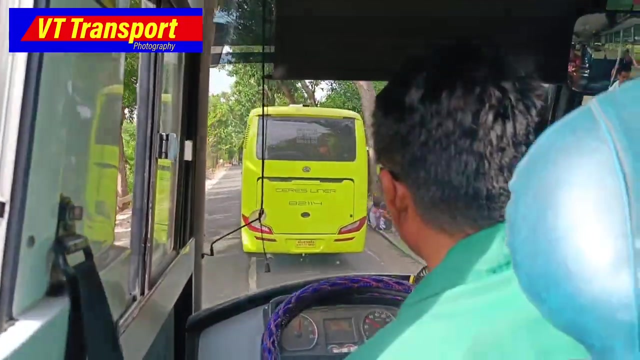 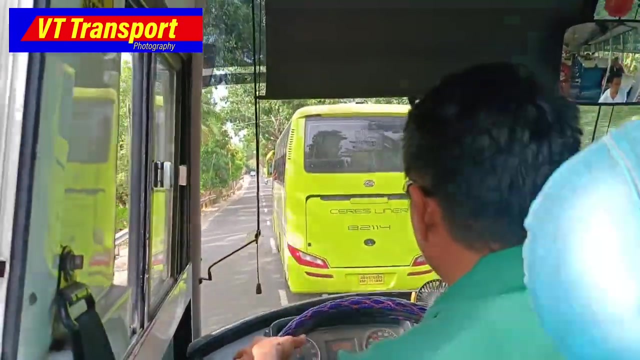 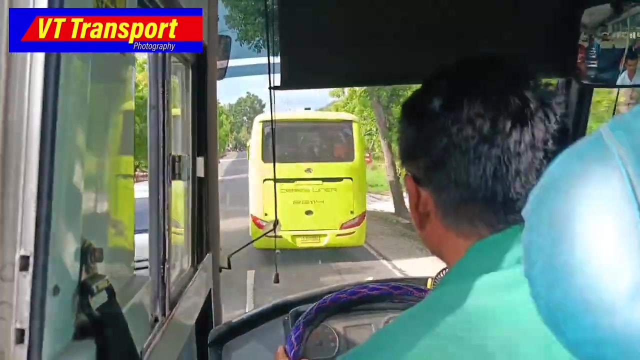 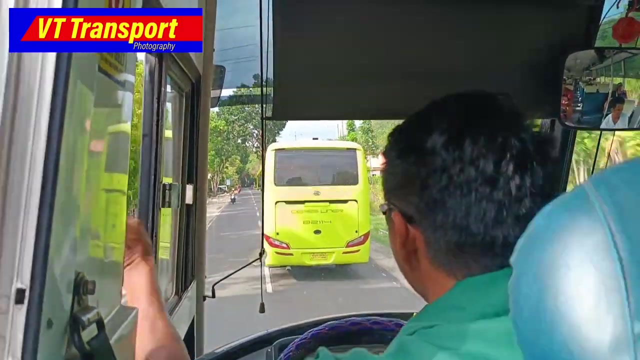 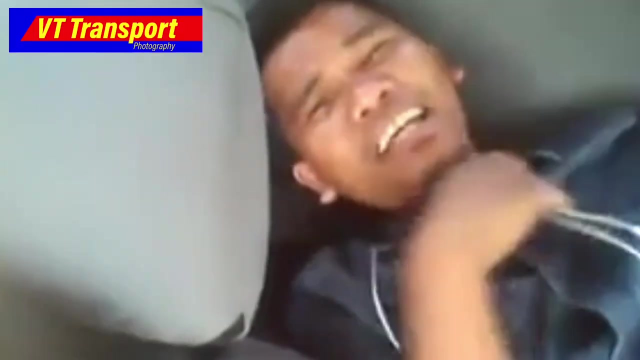 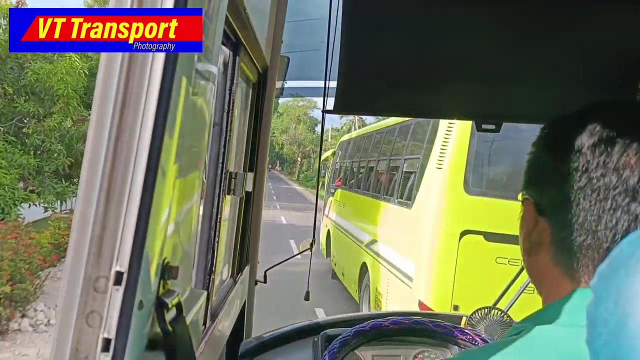 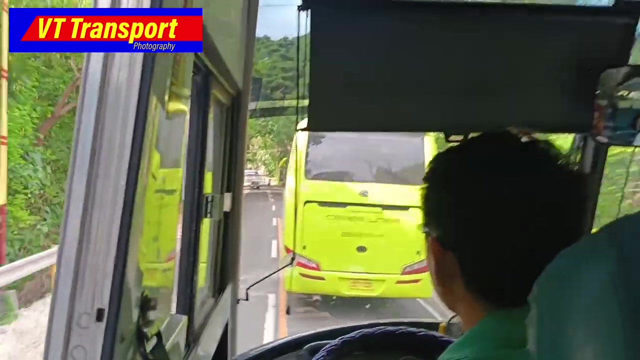 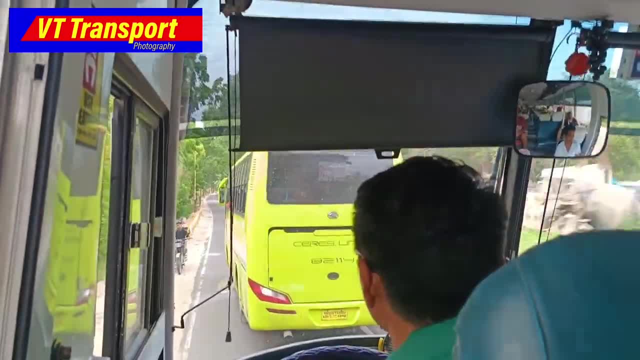 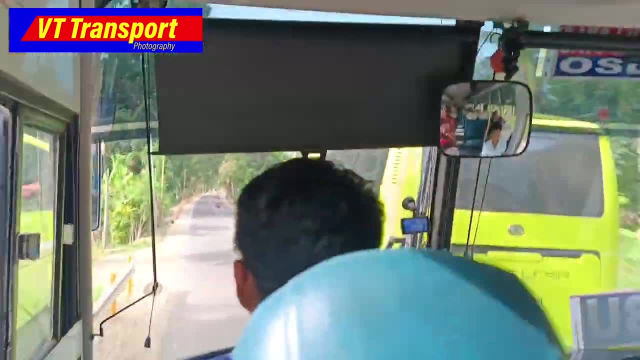 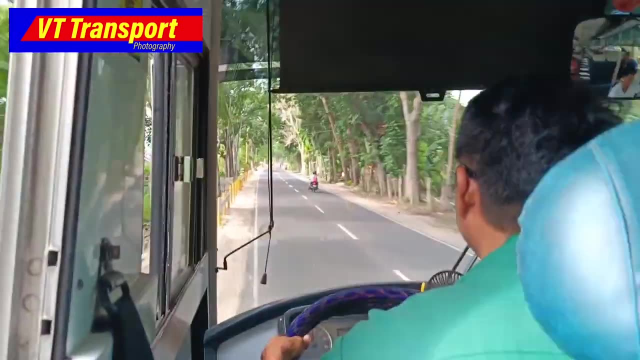 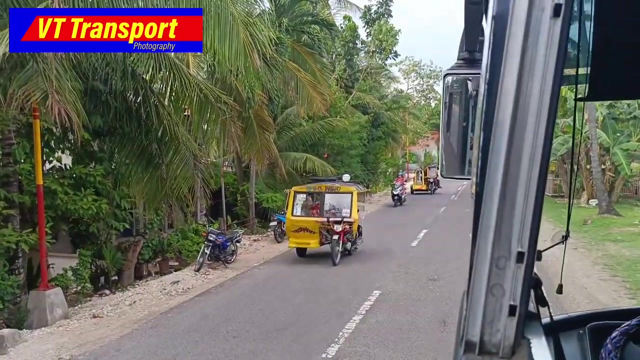 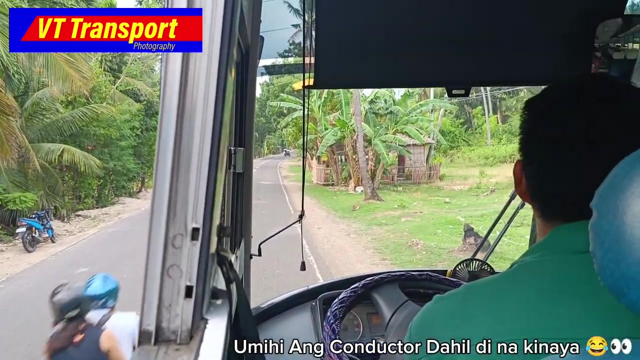 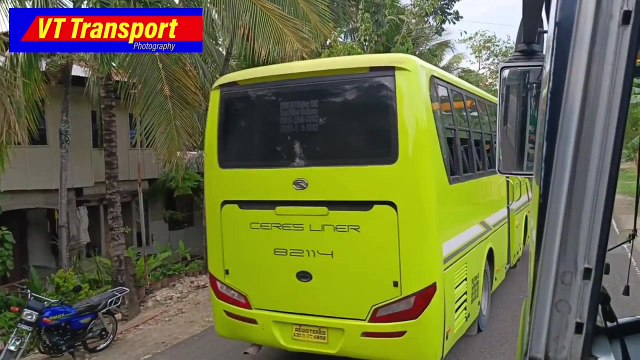 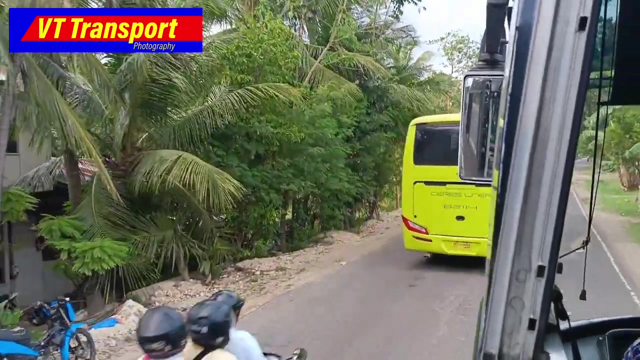 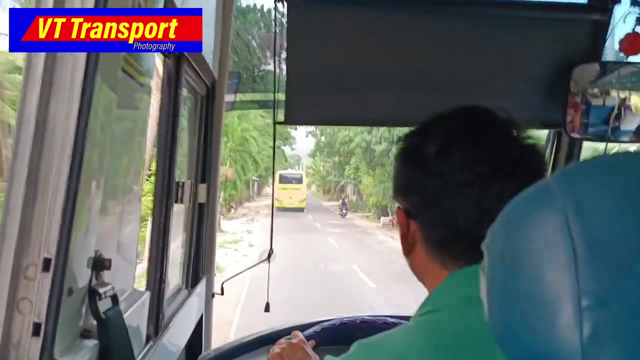 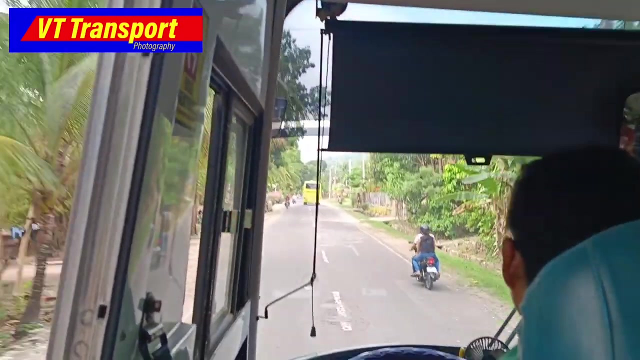 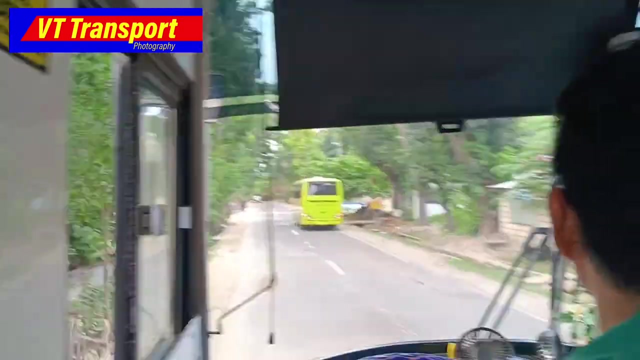 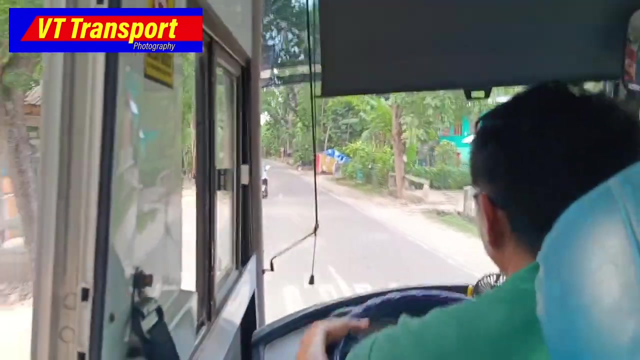 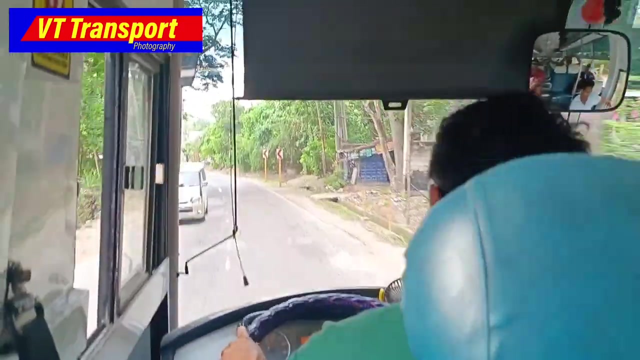 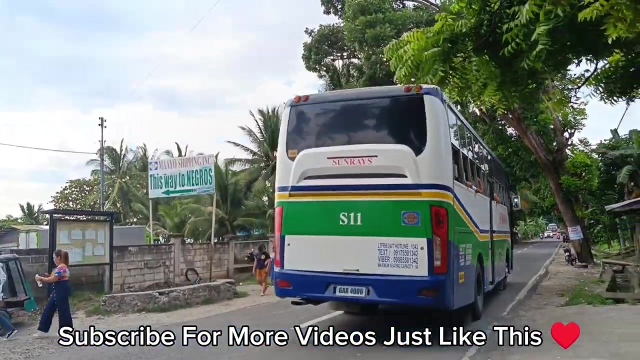 I don't want to be called. I don't want to be called What You're dead. No, No, No, No, Okay, okay, Pass, Remember, remember, Thank you.